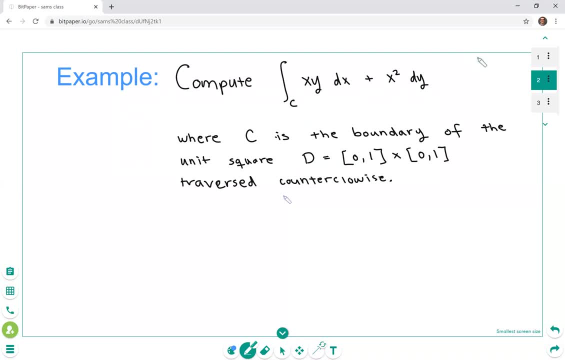 the unit square, So it's traversed counterclockwise. so you can kind of just think: okay, it's traversed counterclockwise, that should be positively oriented. but just to get some practice let's just draw it out. So the unit square here this is like. so this maybe is your y axis. 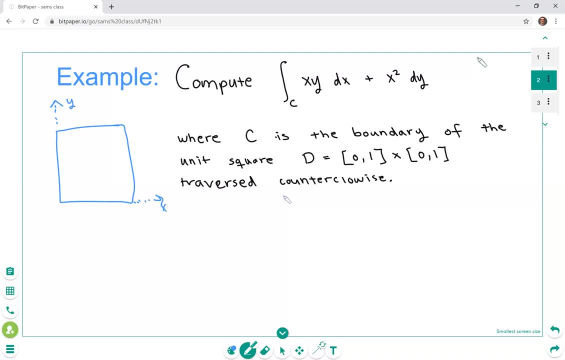 positive y axis and positive x axis. so this is 1: 0,, 1: 1,, 0: 1, and 0: 0.. So this is what it would look like in the xy plane right. So d is the entire unit. 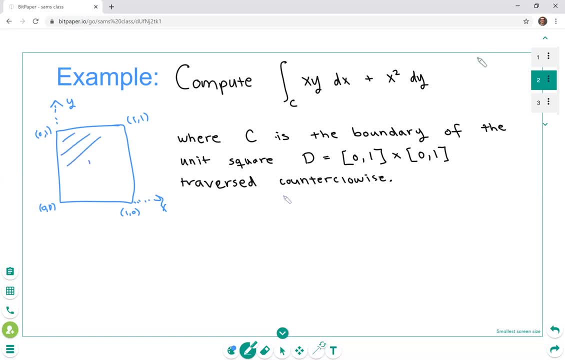 square, It's everything in here, this region. Okay, c and c is the boundary of the unit square, So it's these lines, right, that make up the edges. So this is c and okay. so now you want to picture yourself walking. 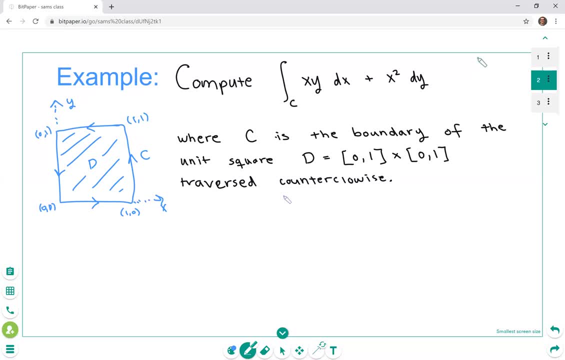 along this curve Is the region on your left? Yes, okay. so this is positively oriented, so we don't have to like multiply by a negative one, We just straight-up use the formula. So what do we need to use the formula for Green's Theorem? 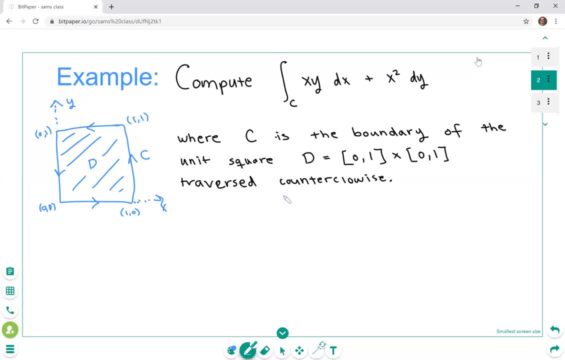 We need to identify what p and q are in this problem problem and then find their partials and take. make sure you subtract them in the right order, right? so p is always the function that is multiplied by the dx. okay, so it's the dx here. 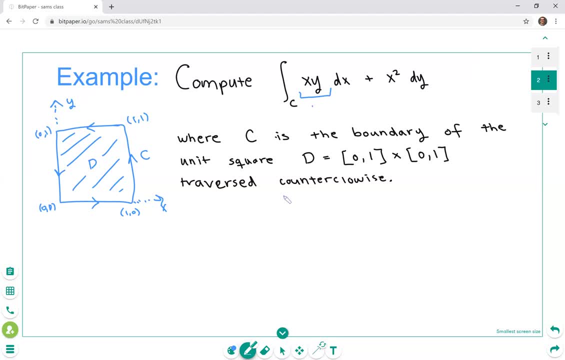 multiplied by the xy. that says: okay, my function p is just xy. and then q is always the thing being multiplied by the dy here. so x squared is multiplied by the dy, nothing else is. so x squared is my function q. okay, so that's how you identify those. then you just have to find the partials and 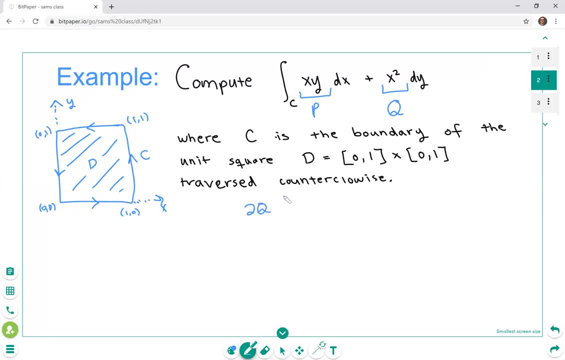 subtract them so to get your integrand your integrand okay. so, partial q, partial y, sorry, x, x. so you always do the opposite, you always do the opposite. so you always do the opposite, so you always do the opposite one. that is one way to remember it. um, so and so, uh, the q is what gets multiplied by the dy. 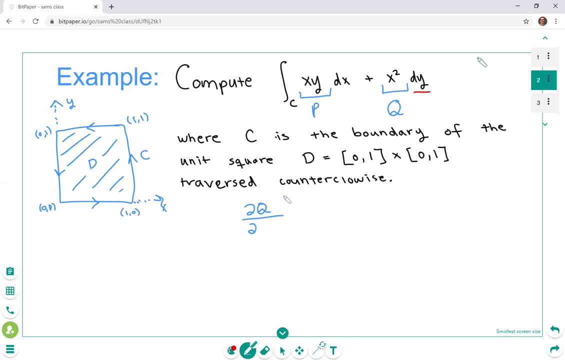 and you always do the opposite one when you take the derivative. okay, so, uh, you want to do partial q, partial x, yeah, so, um, right there, this is of course just 2x, and then again just do the opposite. so p is the function multiplied by the. 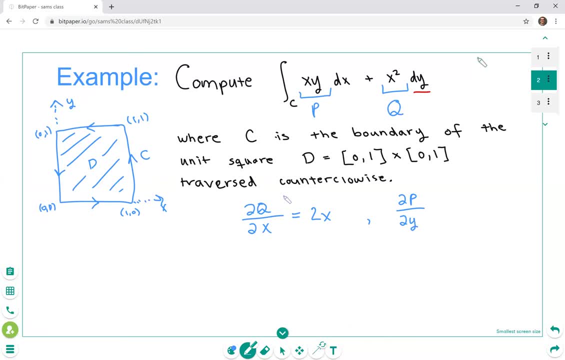 dx, so you take the partial with respect to y, so with respect to y, you just get x. okay, and now, by green's theorem, the integral uh that we're trying to compute is the same as if we just integrated over d the function 2x minus x. so make sure you're always 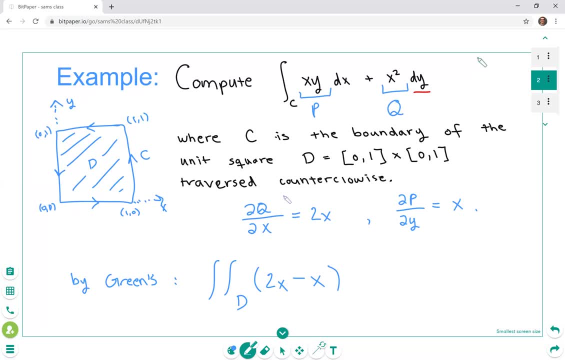 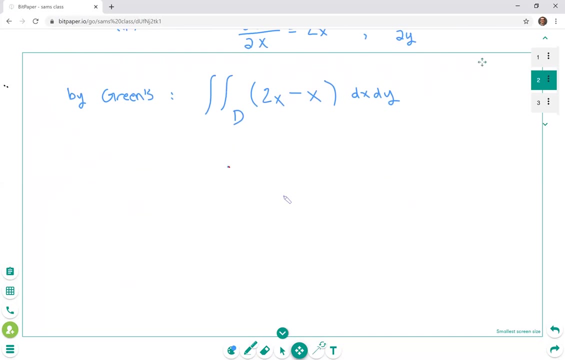 taking the q derivative minus the p derivative. okay, and that's super easy to evaluate right. d is just a square. okay, so we're integrating over a rectangle. um, in particular it's the rectangle zero one cross zero one, so this is just integral from zero to one. 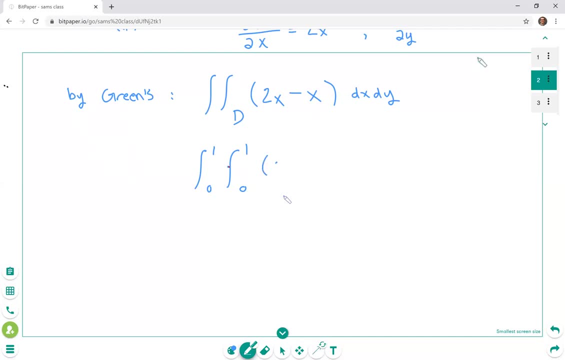 integral from zero to one of. well, 2x minus x, that's just x dx dy, okay. so uh, we get integral zero, one of one half x squared um x is zero to x is one, which of course is just one half. and then integral zero to one dy, that's just one. 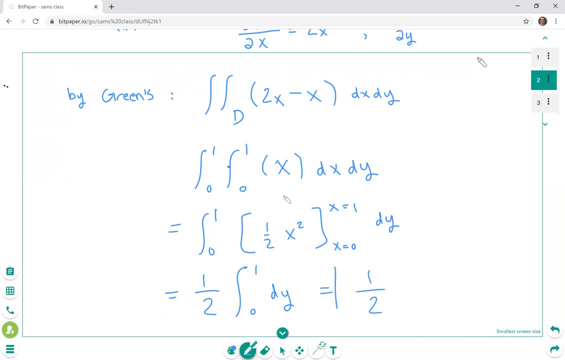 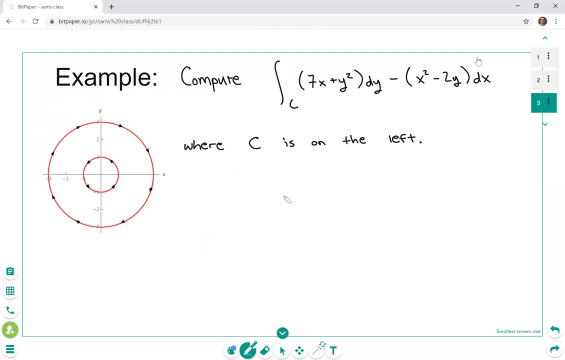 so we should just get one half here. okay, so that's our first, uh, pretty easy example. now let's go on to the next one. so, uh, now we want to compute x squared by x squared integral. okay, again, these uh integrals- we're computing with green's theorem- are always going to look pretty similar. you're going to have something with the dy. 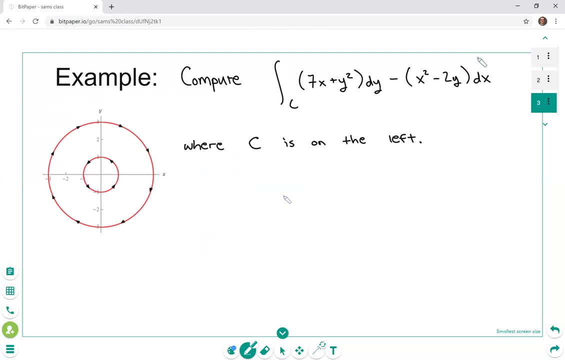 something with the dx over some curve c. right, they're all, they're always going to be- line integrals. we want to rewrite them as a double integral. it's also possible to use this in the reverse direction, where you start with a double integral and then make it into a line integral. 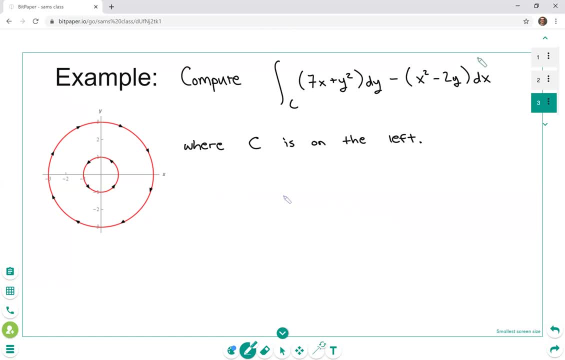 but based on, uh, the kind of conversation that we had in the in the video about green's theorem. well, uh, usually it's a lot easier to just do the double integral than to do the line integral, because, you know, line integrals come up, we have to come up with a lot of parameterizations. 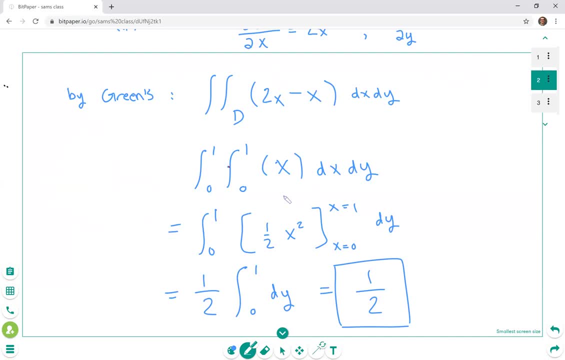 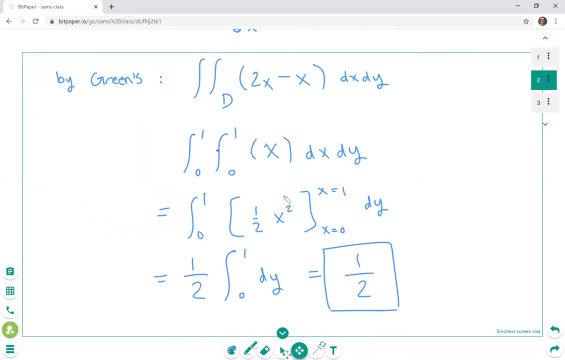 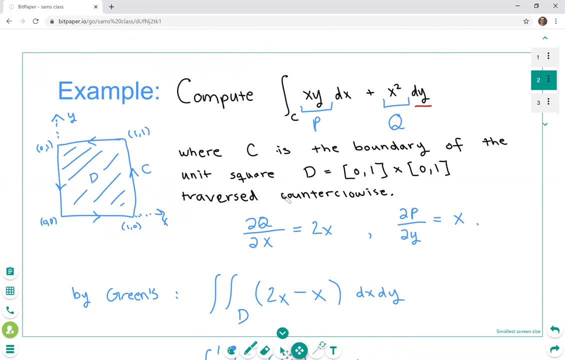 oh yeah, let's actually uh, talk about that for this one. so in this problem, right, let's just first appreciate how easy that was. okay, we just had to evaluate this integral over a rectangle of x, right, dx, dy, okay, so if you were to actually compute this line integral, uh, you would have to. 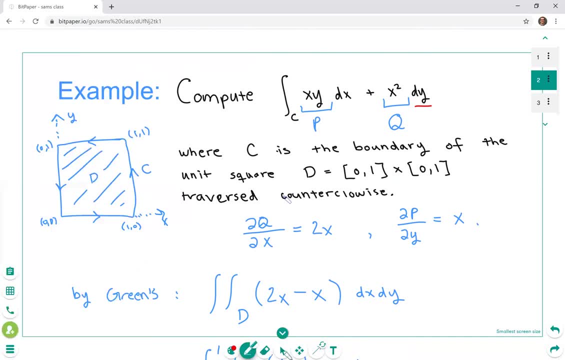 parameterize three curves or right, three lines. right, you have like a c1, right, so they're, they're lines, so they're pretty easy to parameterize, but you'd still have to do four of them. right, you have a c1, c2, c3, c4, okay, and then for each of those you would have to. 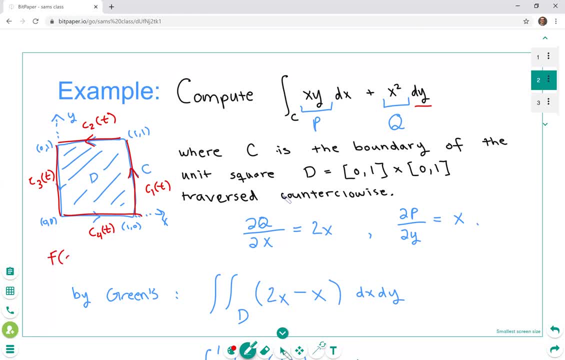 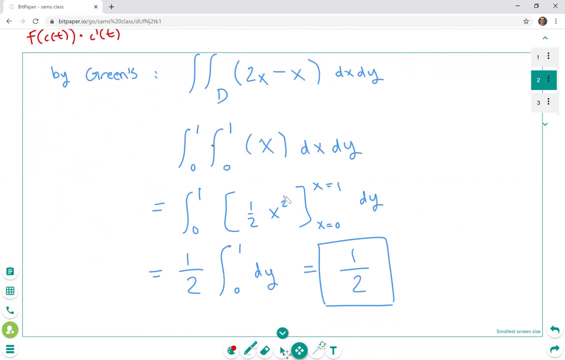 compute right, um, right, f of c of t dotted with c, prime of t, right? so it's just gonna be a lot of computation if you were to do it as a line integral. so we saved a lot of time using green's theorem here, okay, so hopefully that gets you to appreciate this theorem a bit. okay, uh, same thing. 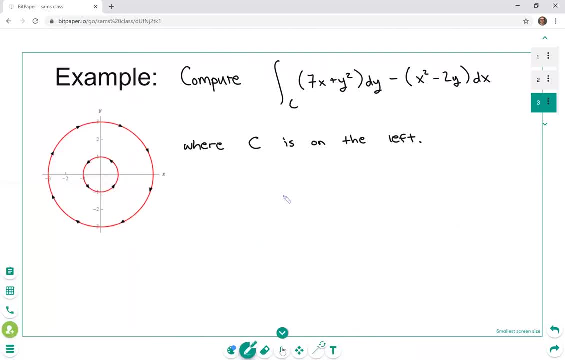 here, right. if we were to try and do this line integral without green's theorem, we'd have to characterize um two circles here, which sure is not bad. you just use sine and cosine um, but you, you'd have to do two integrals. uh, you have to split it up, right, so so yeah, this is our curve. 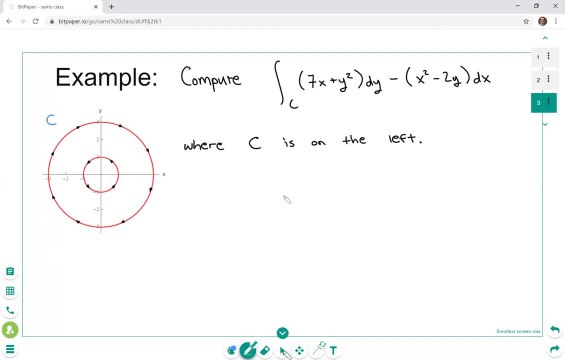 c on the left here, and first let's just think about our. no, sorry. first thing i just want to note here is that the line integral is written a little backwards right. we have the thing multiplied by dy first, actually um, so we're used to it the other way. so 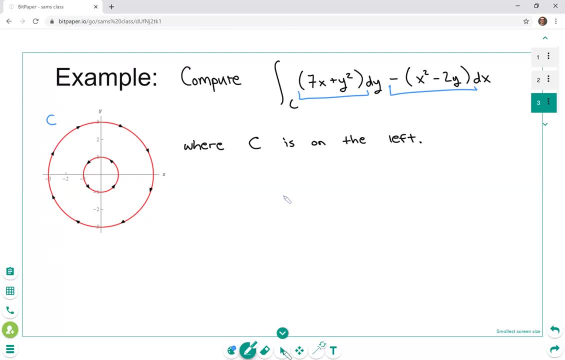 this is why i pointed this out earlier. whatever is multiplied by the dy, that is what you call q. whatever is multiplied by the dx, that's what you call p. okay, so our p and q are kind of swapped here. um, usually we write the dx first and then the dy, but it's the other order. okay, so now, uh, before. 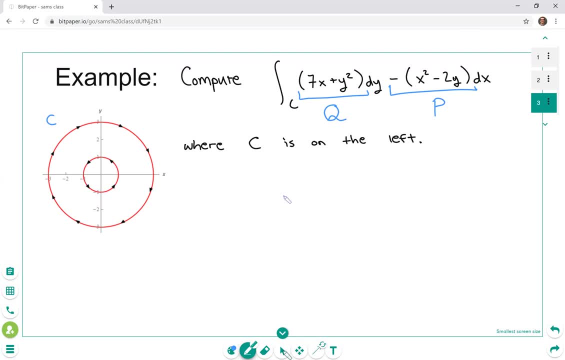 i talk about anything else. um, why don't you pause the video here and decide whether this curve c is positively oriented or negatively oriented? okay, now that you've unpaused. so first you probably want to just identify what region d we're looking at, and so there are some different regions. you can maybe think of this curve in. 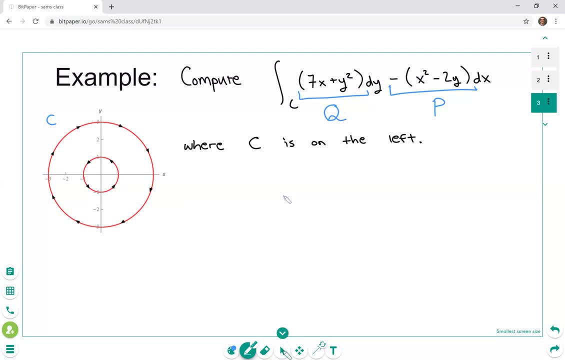 closing um. so the curve c is the region d where we're looking at, and so there are some different regions that we can think of. the correct one in this case is the donut right. what's inside here, and this circle in the middle is actually going to make a hole in the region. we don't include that. 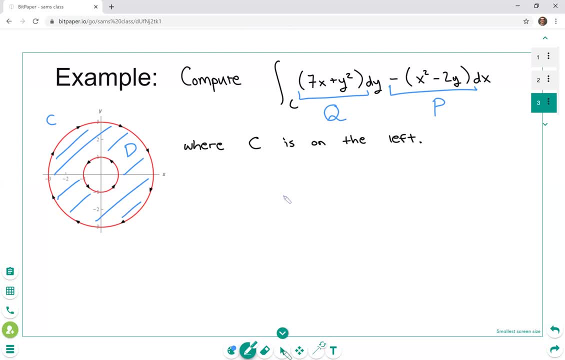 because if you were to instead include kind of this whole area, then you would have to also include what is outside of the curve, and that would be right in unbounded region, if you think of what's outside the circle of radius three, and so this is a circle of radius three and radius one. this is if you. 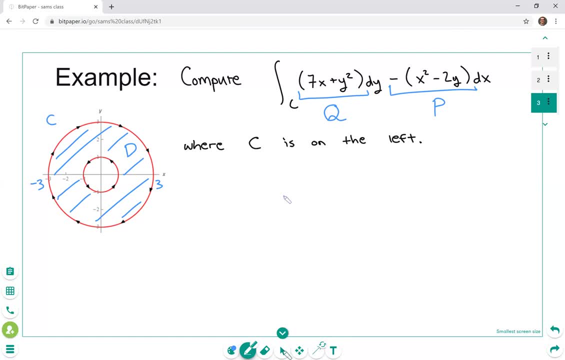 can't see that? uh, just from the picture that i pasted here. um, the inner circle is radius one, outer one is radius three. so, uh, this is the region d, it's the donut region, because otherwise we'd have an unbounded region and we don't want to deal with an unbounded region. so how do we determine if? 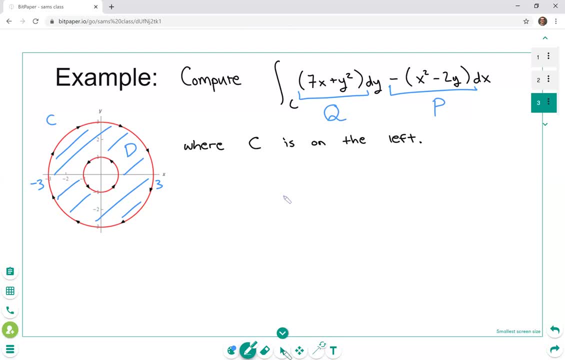 this is positive or negatively oriented. well, uh, take your computer, throw it on the ground and walk on your computer screen. uh, no, so you just visualize it, um. or you could maybe even use your fingers, uh, to walk along the computer screen on this, if that helps for you. but if you want to, 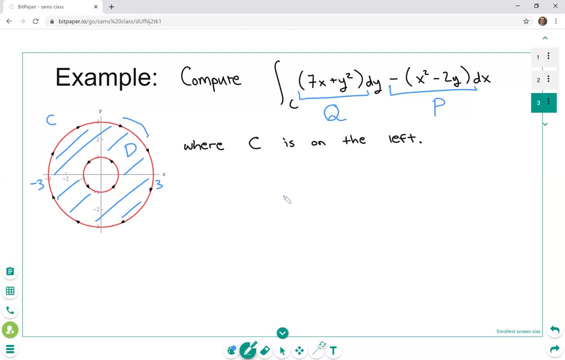 think of like a little guy walking along this curve and the region d here is on the right, okay, no matter which one you choose, right? if you're walking around the circle of radius three, it's on your right, and also the one on the inside right the region is on your right, okay. so this is negatively oriented. 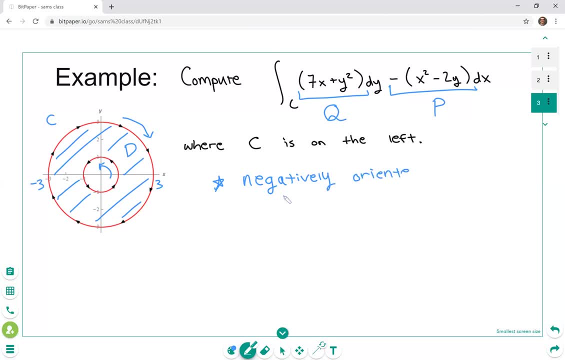 okay, now that we have that, why don't you pause the video again and just try and compute this entire? just do the entire problem computing that integral. make sure to use green's theorem. yeah, compute this integral on your own and then unpause when you're done. 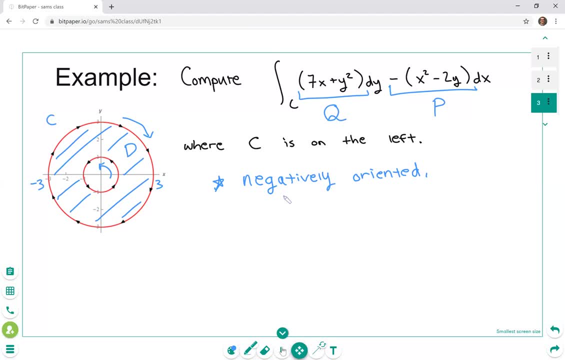 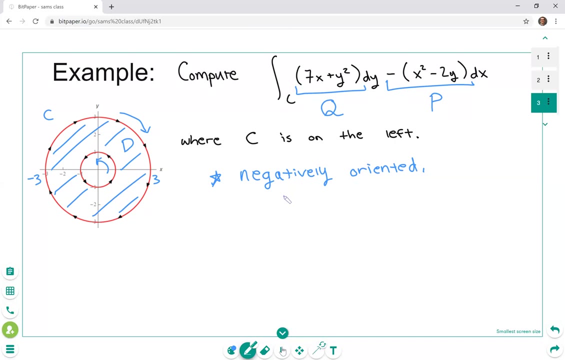 okay, now that you have computed the integral on your own. so i believe you should get 40 pi. so if you got that, then maybe you're good. but uh, i'm gonna work out the entire problem here. so we have p and q, so let's just compute the partial derivatives right away, that's. 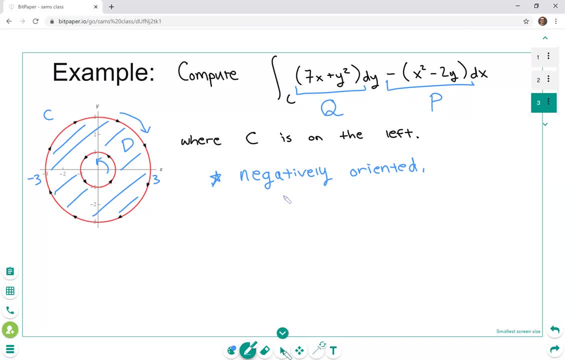 what we're going to need in order to use the green's theorem formula. so partial q, partial x is what we're doing, right. q is multiplied by the d- y, so we take the partial with respect to x. that's just seven. y squared goes to zero. okay, partial with respect to x. 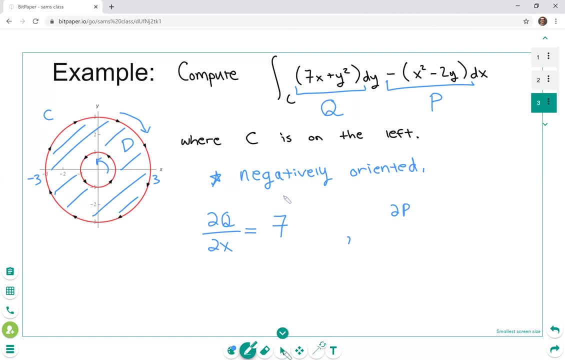 a little review there now. partial p respect to y. all right, these partial derivatives are never gonna go away, okay, so, uh, we have to include this negative here. this negative is part of p, because in the formula we have p, d x plus q d y. okay, so there's not normally a negative there we have. 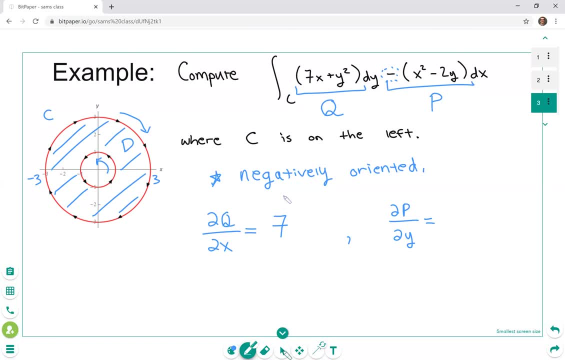 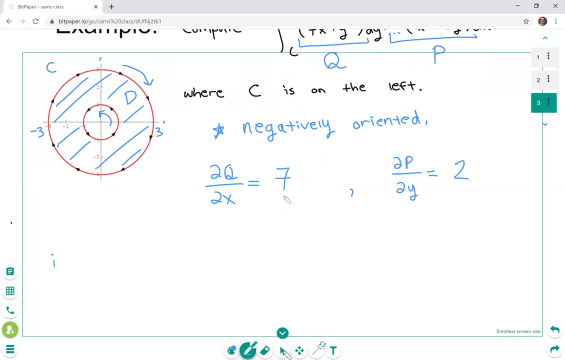 to include that. so we get: uh, negative x squared plus two y derivative, with respect respect to y, is plus 2. okay, so our integral becomes. so the line integral we get we ought, by Green's theorem, is the double integral over D of well, Q, DX is. 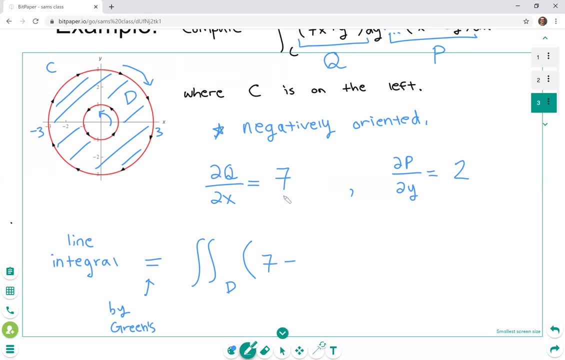 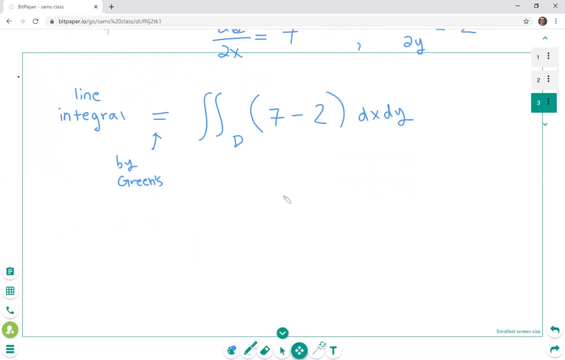 7 minus P dy, which is 2. okay, so we're just integrating the function 5 over D. so there are a couple ways you could do this right. since you're just computing the double integral of a constant 5, you can just take 5 and. 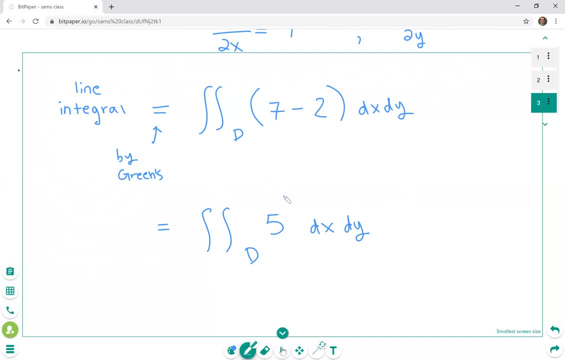 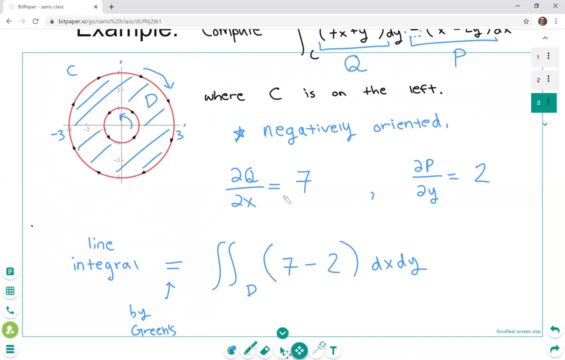 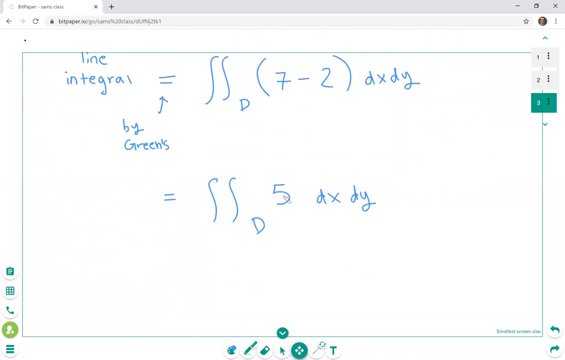 multiply by the area of D. okay, so maybe you geometrically compute the area of D here just using the area of circles, and then you know that becomes your integral. you just multiply by that, that by 5 and that's your integral. so another way to do this here is to convert to polar right? so since we have circles in 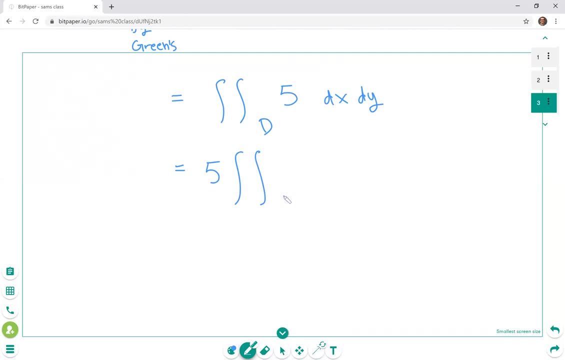 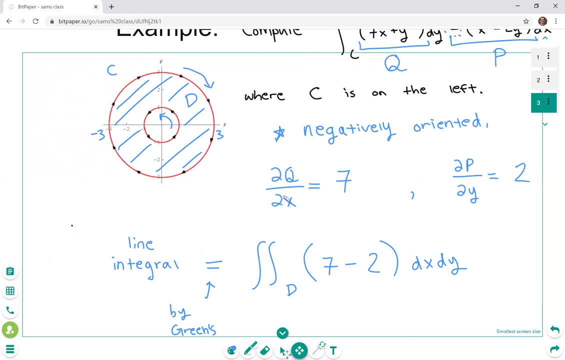 the mix for a region D. why don't we convert this to polar? theta just goes from 0 to 2, pi and R. well, we have a hole in the middle. this is a donut, so R goes from. it starts at 1 and goes to 3. 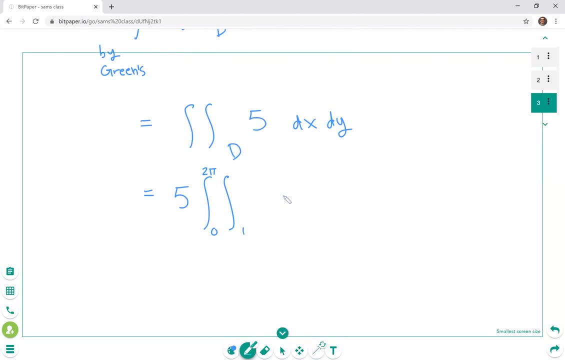 and then remember the Jacobian for this transformation. if you're doing the polar coordinate transformation, the Jacobian is R, dr d theta, right, sorry, the Jacobian is just R, right? so you have to multiply by R and then DX dy go to dr d theta, okay. so this is our integral. we have 5 and 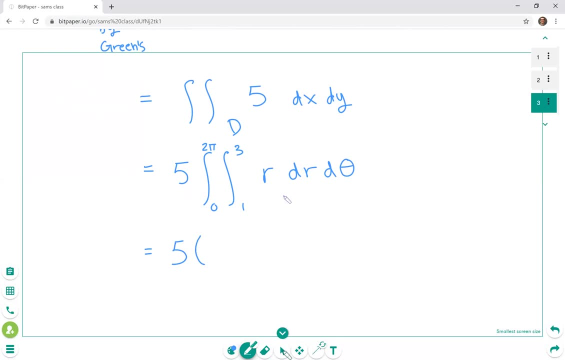 times right this function. here it's just R. this is independent of theta. so the integral 0 to 2 pi of D theta, that just multiplies it by 2 pi, and then integrate R- dr, that's 1 half R squared. okay, so this becomes 10 pi times 9 halves minus. 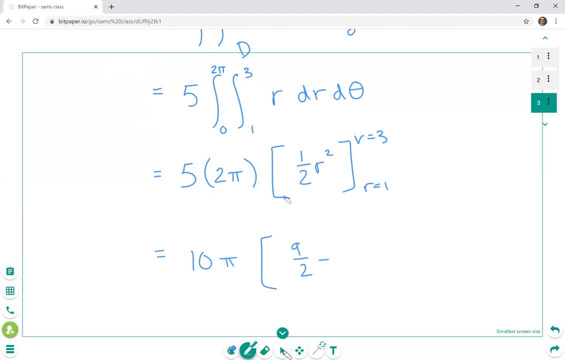 times 9 halves minus 1 half, which is 8 halves, in other words 4. so 4 times 10 pi gives us 40 pi.